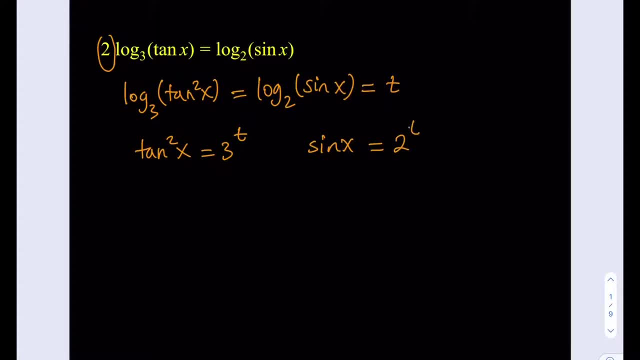 And sine x equals 2 to the power t. Okay, Now I can write tangent squared as sine squared over cosine squared, Which can be written as sine squared over 1 minus Sine squared. Okay, This is good, because now I can replace sine x with 2 to the power t. 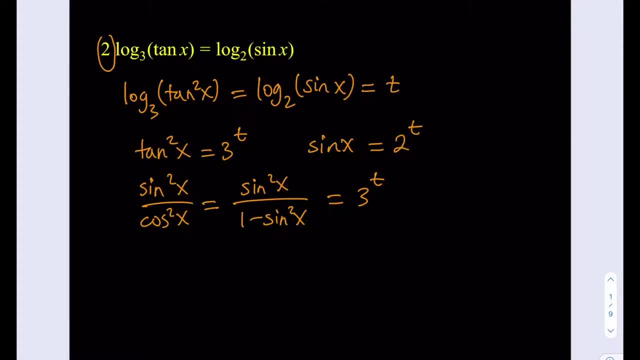 So that's going to give me 2 to the power t squared, which is 4 to the power t Divided by 1 minus 4 to the power t. So this is what I did, Because sine x is 2 to the power t. 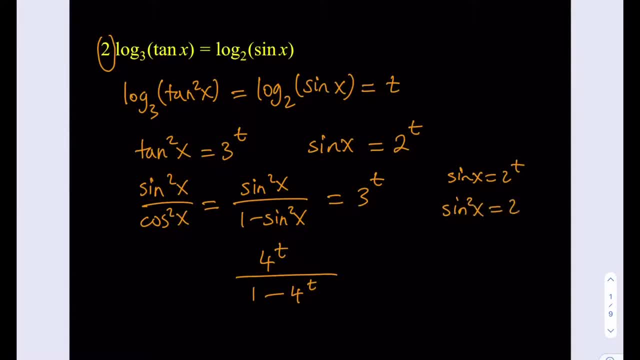 Sine squared x is going to be 2 to the power t squared, Which is 4 to the power t. Okay, And this equals 3 to the power t. Now we do have an equation in one variable, which is pretty good. 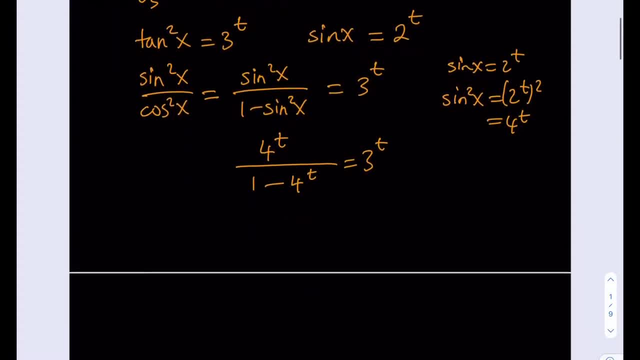 Even though the bases are different. we're going to take care of this. So let's go ahead and cross multiply this expression first. So we're going to be getting 4 to the power t equals 3 to the power t multiplied by 1, minus 4 to the power t, times 3 to the power t. 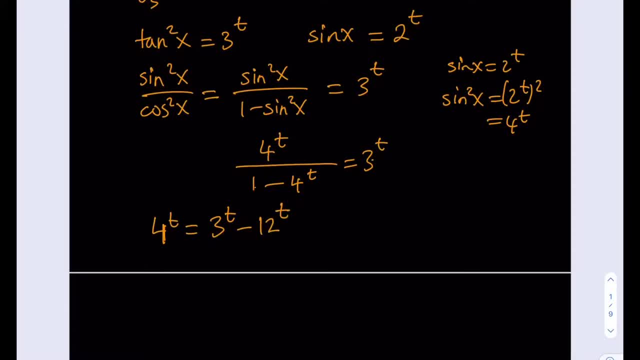 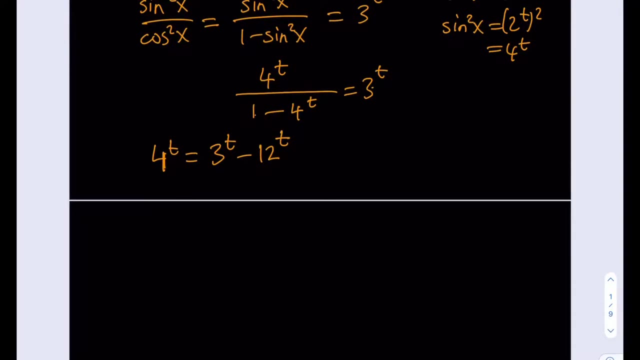 Which is going to be 12 to the power t. Okay, Alright, so we want to simplify this a little bit so that we can kind of make some comparisons. So what I'm going to do is I'm actually going to divide everything by 4 to the power t. 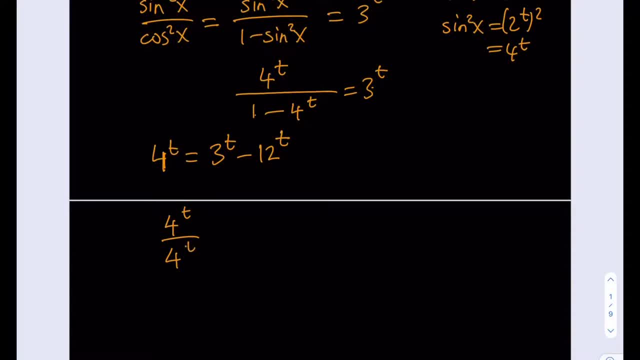 So it's going to look like this: 4 to the power t divided by 4 to the power t, Which is equal to 3 to the power t, minus 12 to the power t divided by 4 to the power t. Okay. 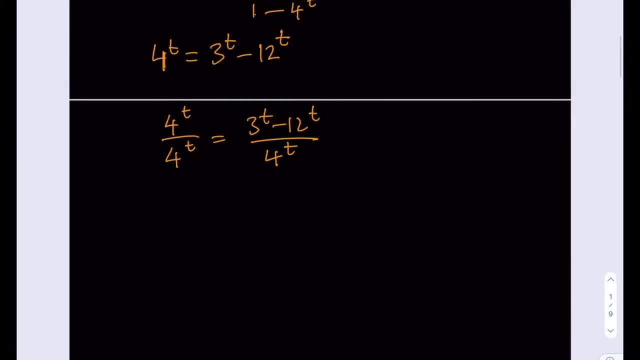 Obviously, I'm going to have 1 from the left-hand side- right, That's going to be a 1. And the right-hand side. we're going to get 3 over 4 to the power t, because they have the same exponent. 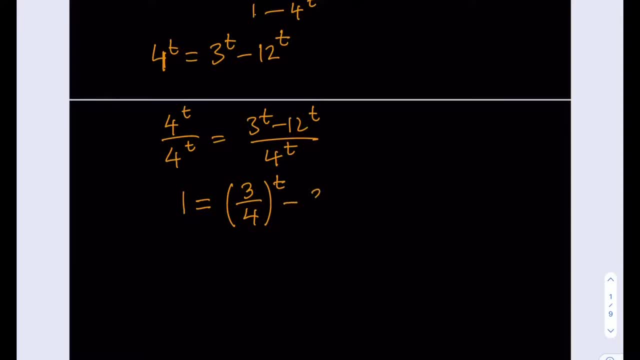 Minus. now they have the same exponent, so I can just divide the bases and that's going to be 3 to the power t. Okay, In this form this is not very helpful. So what I'm going to do is I'm actually going to isolate 3 over 4 to the power t. 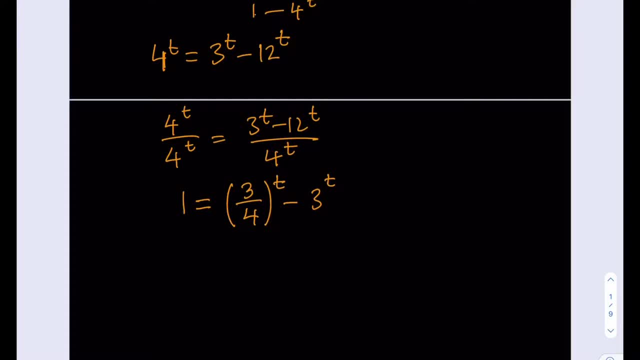 So I'm going to add 3 to the power t to both sides, So that's going to be 3 to the power t plus 1.. And 3 to the power t plus 1 is equal to 3 over 4 to the power t. 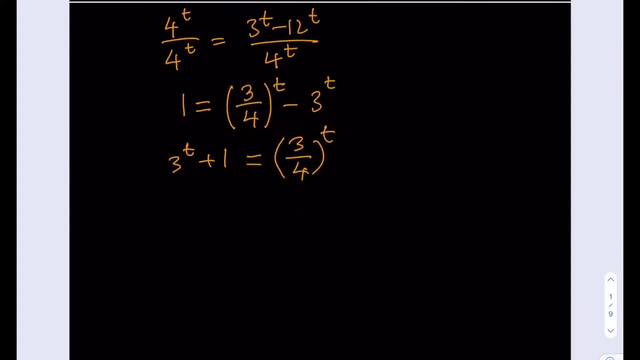 Okay, Now, this is good because, as we know that, 3 fourths to the power t is a decreasing function Because the base is less than 1.. Right, And this is an increasing function because the base is greater than 1.. 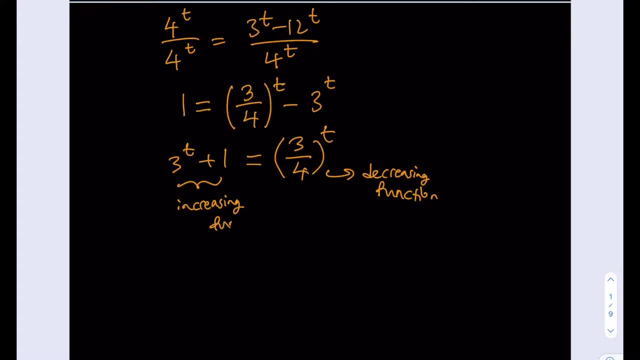 Okay, Alright. So what does that mean? You have an increasing function. You have an increasing function like this and you have a decreasing function like this. That means they're just going to intersect at a single point. So we can actually find that point by inspection. 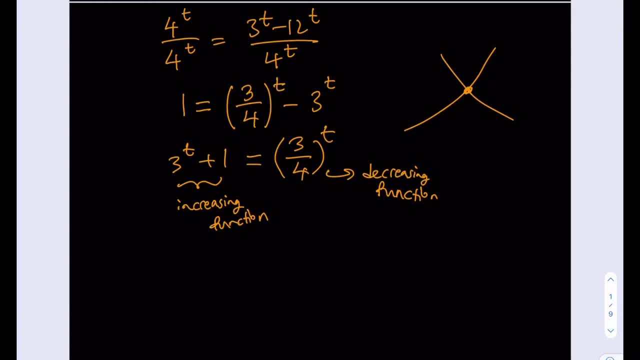 And that shouldn't take too long. If you just try some small integers here, you're going to notice that t equals negative 1 is the only solution, Because if you replace t with negative 1, you're going to get 3 to the power, negative 1 plus 1 on the left hand side. 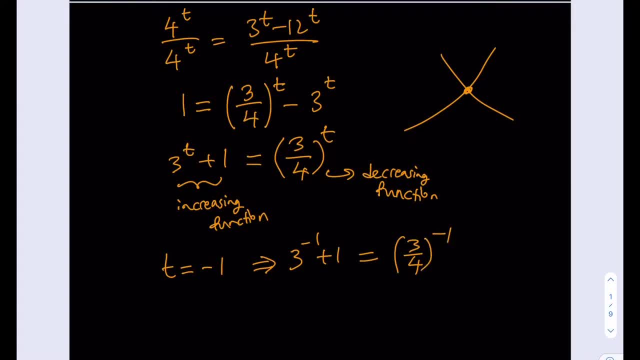 And 3 fourths to the power negative 1 on the right hand side. This is equivalent to 1 plus 1 third, which is 4 thirds, And the reciprocal of 3 fourths is also 4 thirds. So this checks. 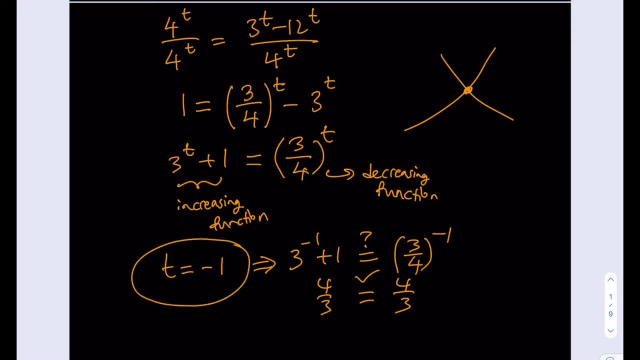 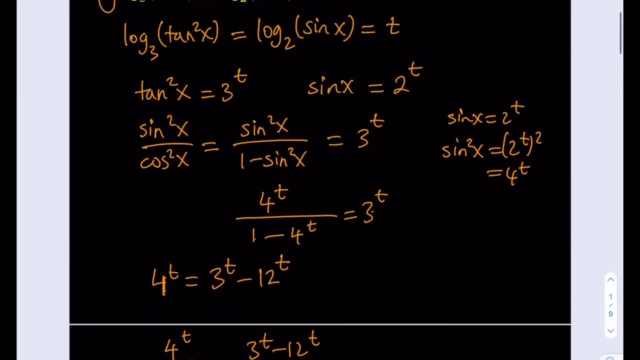 Okay, So t equals negative. 1 is obviously a solution, So let's go ahead and use that. How do we use that? Well, if you go back to our initial assumption that we said that sine x is equal to 2 to the power t, 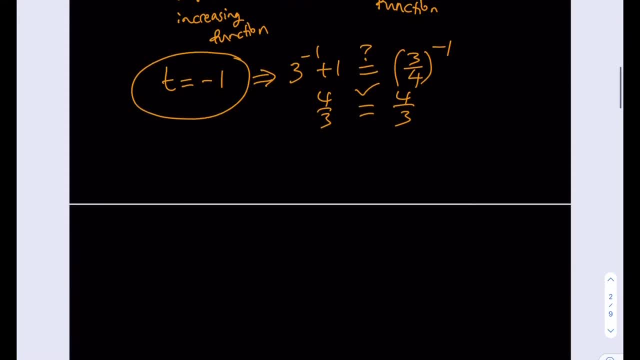 Right. So we're going to go ahead and replace the sine x with 2 to the power t And, as you know, 2 to the power t is equal to 2 to the power negative 1.. Because we just found the t value to be negative 1.. 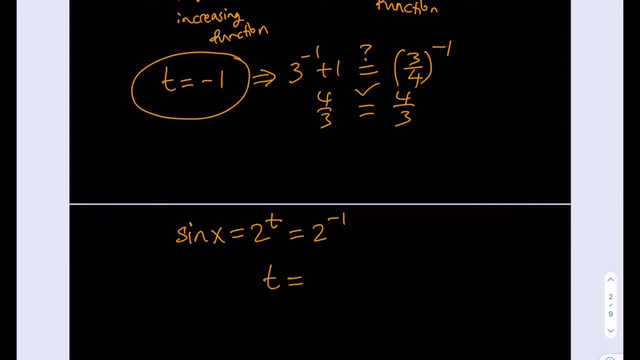 And from here we're actually going to be getting t equals negative 1.. Right, And now t equals negative 1. Meaning that, well, actually we don't really need the value of t, But we just have. from here we get that sine x is equal to 1 half.